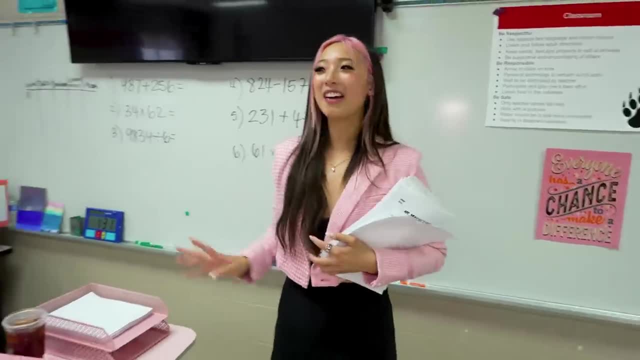 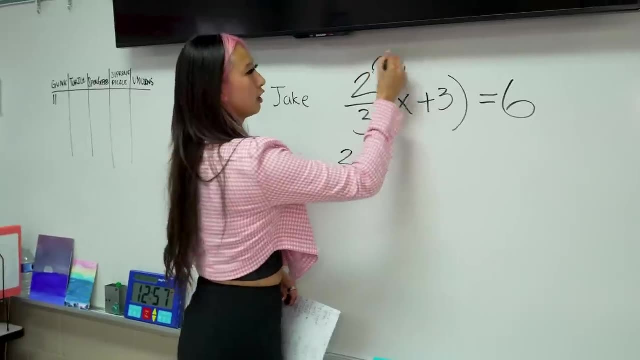 We are at a middle school and I'm about to teach a math class. I put together a test with math problems ranging from simple addition and subtraction to more complex long division and multiplication problems, And my mission today is to get every one of these kids to pass, because 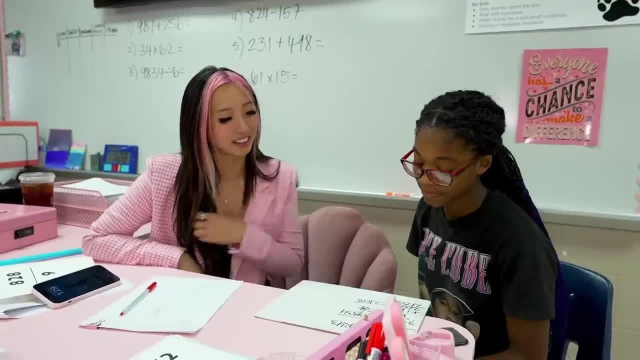 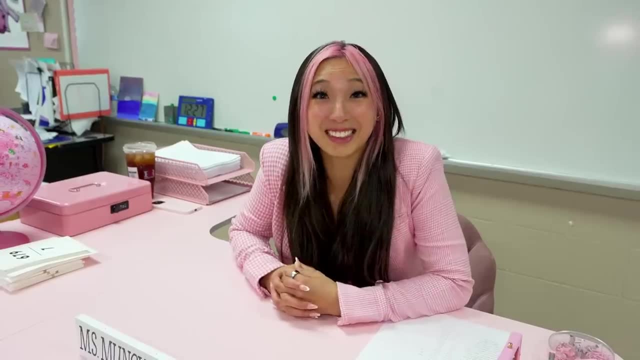 if a single one of them fails, I have to get a tattoo. So I need to do whatever it takes to make sure every student is prepared to pass. Let's see how they do. This is the first math class I've ever taught. Middle schoolers are really scary to me. You can hear them. they're coming. What if I don't? 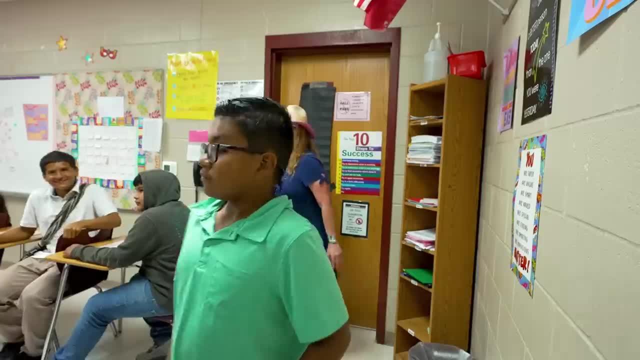 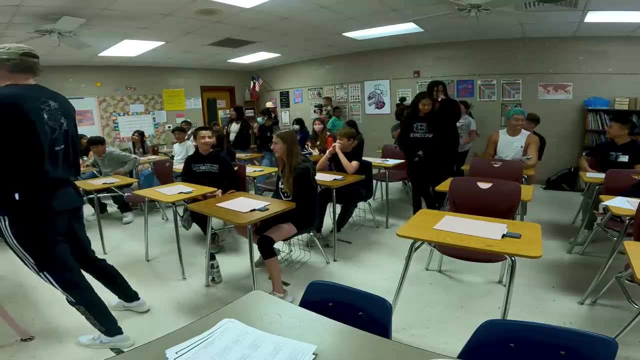 prefer Welcome class. By the way, this is Ms Carol. She was kind enough to let me teach her class, so I hope I don't fail her students. As the kids came in for class I realized a few of my students looked familiar. What up boys. But I wonder who's going to sit next to me. I am Back when I was in. 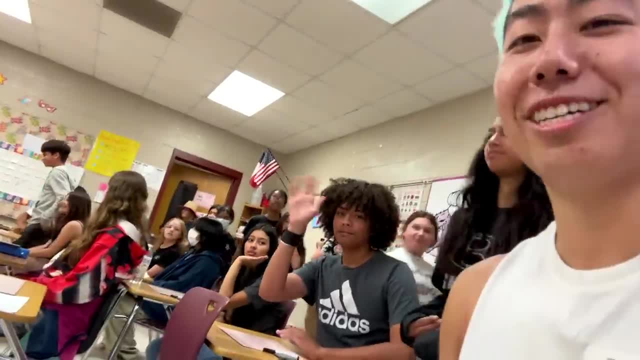 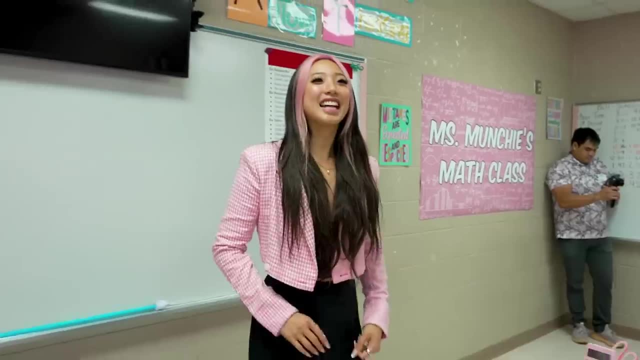 middle school, nobody wanted to sit next to me. Well, you have friends now. Hey, what's up? This is a full class. Hi, everyone, Hi, Hello, What's up? I'm Zach. Zach, stop talking in class. I'm trying to make friends. I had no. 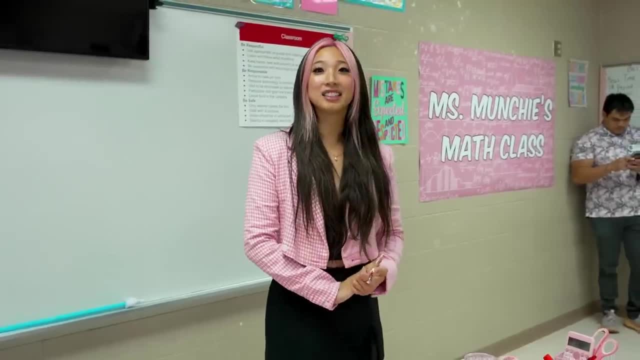 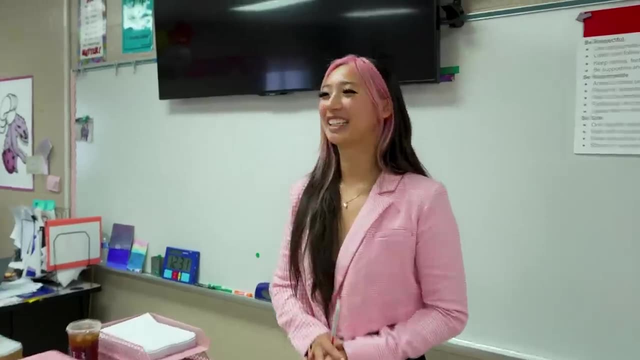 friends in middle school. Before I knew it, it was time to start the class. I guess we'll start with roll call. Say fun fact about yourself. You can all call me Ms Munchie. My fun fact is I play the violin. 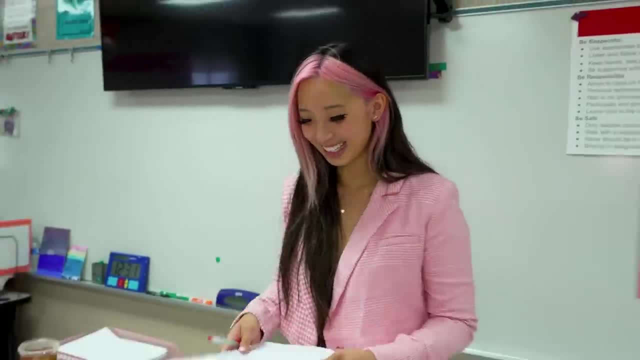 That is really fun. It's so I like to dance. Oh good, Pretty soon I knew everyone's names and started to feel a lot more comfortable. I feel like I already learned so much about my students. Benjamin, I'm. 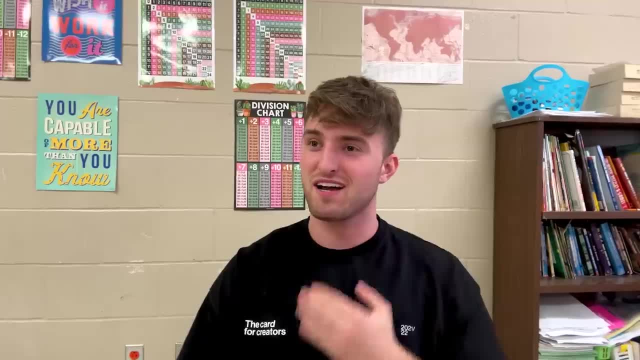 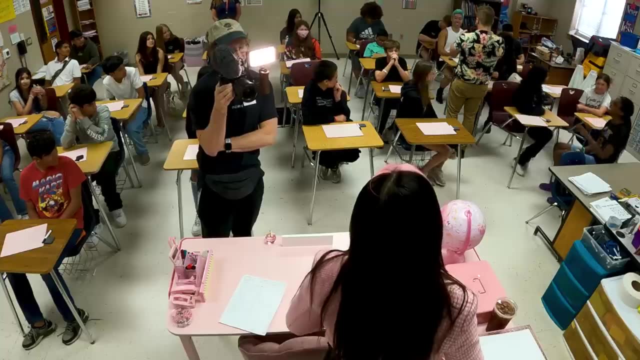 subscribed to Ms Munchie. Yay, Jake Riley, I'm an artist. I never finished my artwork, That is true, Great. Did I miss anyone? My name's Zach and I'm dating Ms Munchie. Oh, Things are off to a pretty awkward start. We're. 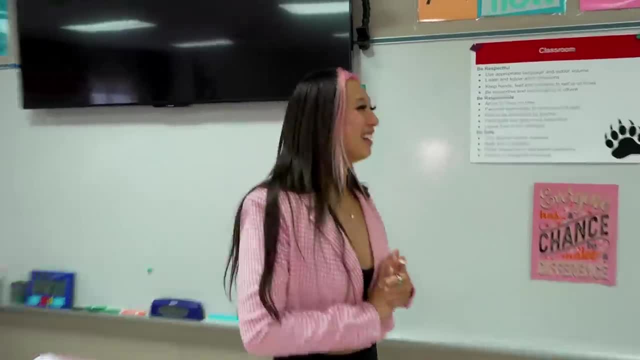 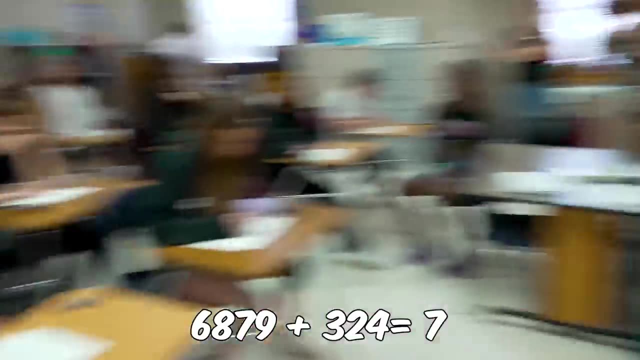 gonna start off with a pop quiz. Huh, Woo, Not many kids were that eager to participate. Okay, who's got the answer? Oh, okay, 7,100.. Close, but that's not it: 7,200.. Yay, congrats. 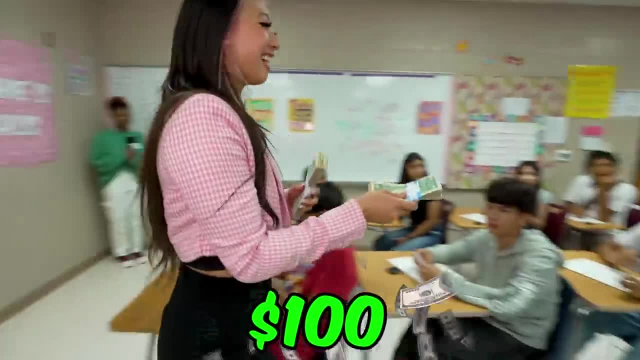 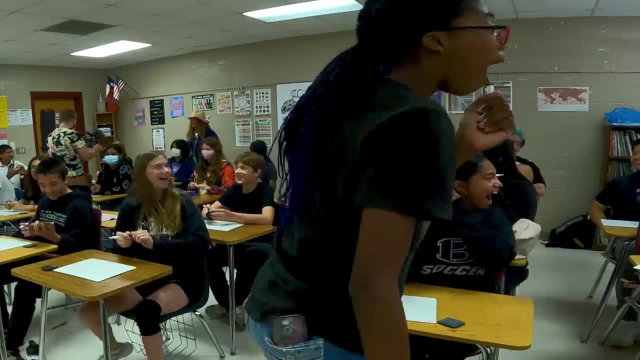 Little did they know. I had a plan to keep them engaged. Here's a hundred dollars. Here's a hundred dollars. Thank you for the money. Thank you for participating. Aside from wanting to keep the students engaged, I'm hoping this will serve as a little gift for passing the seventh grade. I should say that you. 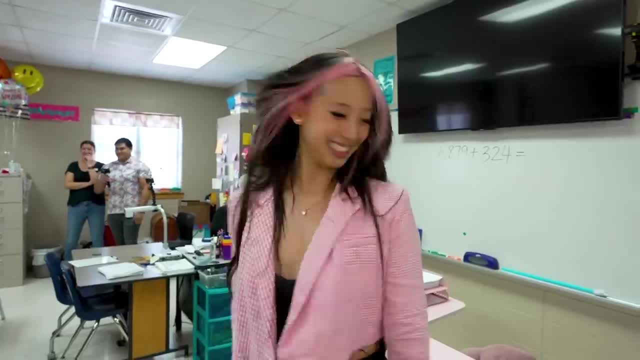 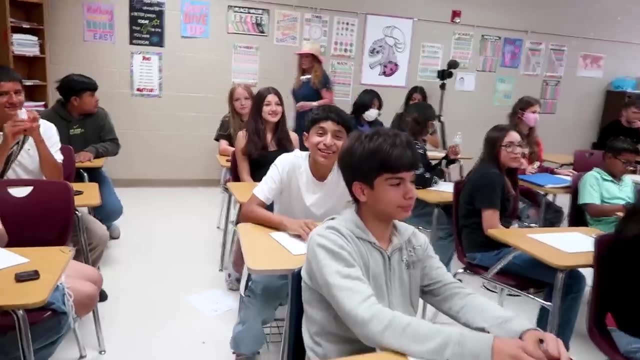 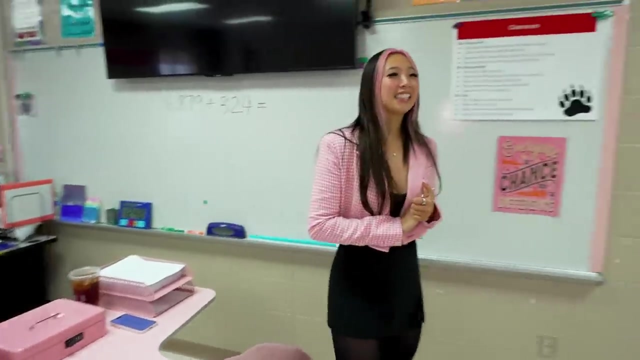 get problems wrong. but just because you participated, congratulations. I don't think they were expecting money. I think the most difficult is getting everybody to participate, getting everybody to have fun. At the same time, I need to make sure they concentrate so they can prepare for the final test. All right, everyone In this class. 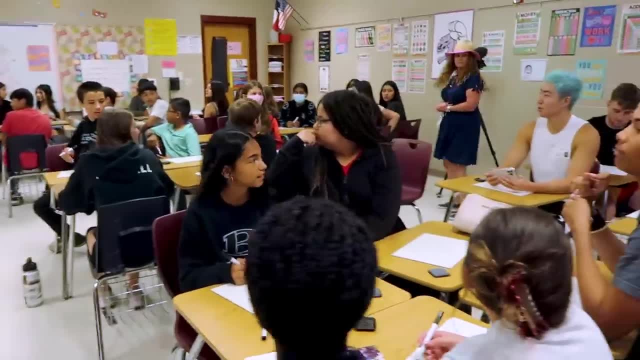 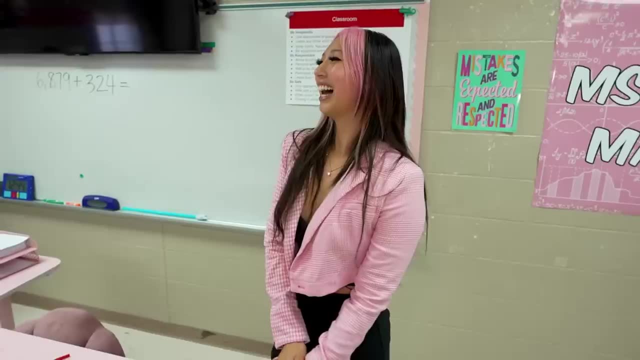 I am preparing you guys for a big test. Wait, what happens if you don't pass? I have to get a tattoo. and if every single person doesn't pass? so please pass. But after telling the kids about the stakes, some of them thought it was funny for me to get a tattoo. Wait, do we get to pick a tattoo? Hold on. 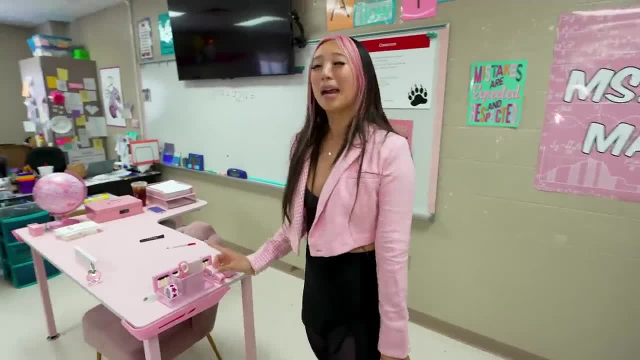 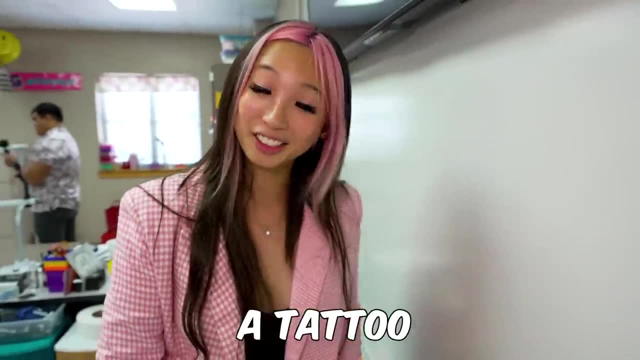 Tattoo, tattoo. Are you guys saying you guys are purposely going to fail? Yes, No, no, no, we don't fail in this class. Maybe I shouldn't have told them. I don't want a tattoo. To get the focus back on passing the test. I decided to make things competitive. 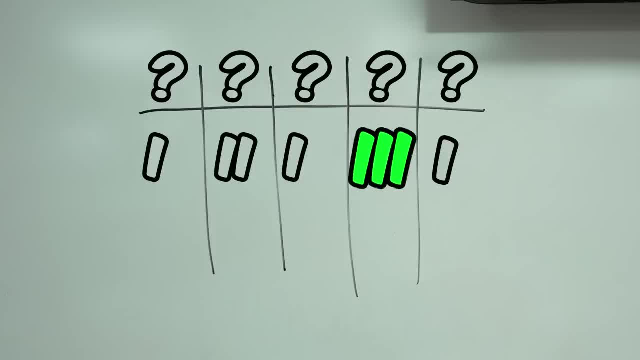 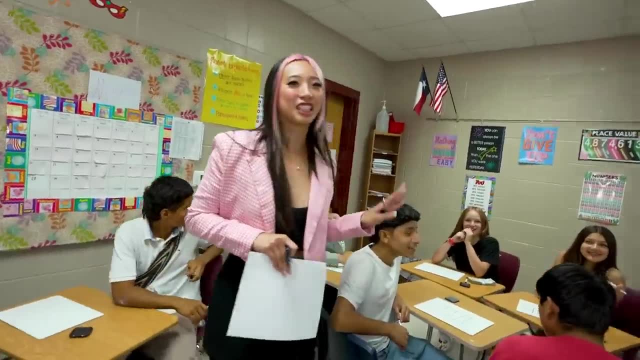 We're going to do a bunch of questions and the first group to make it to three points wins. What's your guys' group names? Gum Gum Team, Gum Team, Turtle, Team Turtle. I like that, That one's cute SpongeBob. 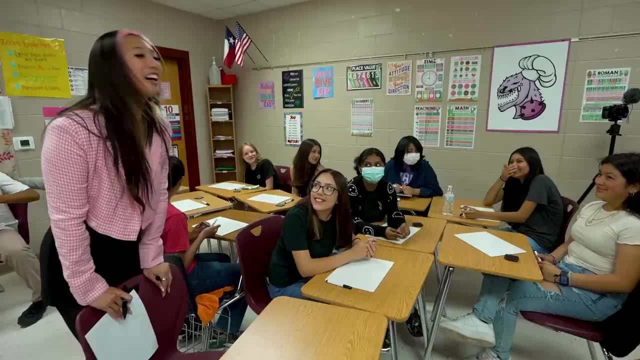 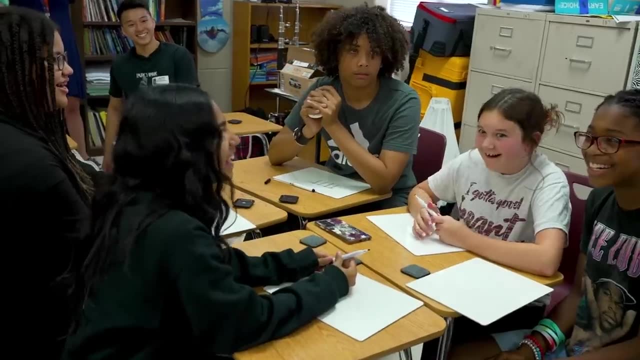 SpongeBob. What inspired that? I don't know. SpongeBob, Supreme Pickle, Supreme Pickle, Unicorns, because the room is pink, I love it. Are you guys confident? Yeah, Yeah, duh, There you go. But then I noticed a couple of students were slacking off. Oh, 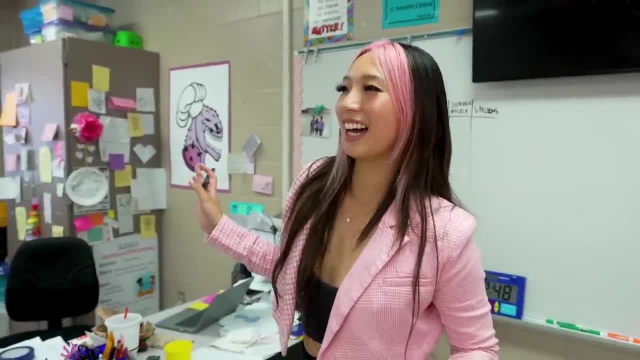 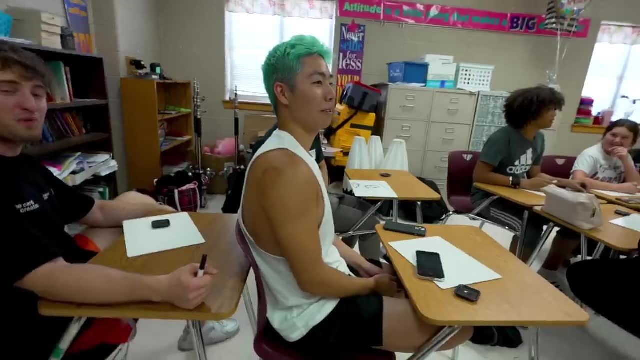 are you guys a team? I haven't paid attention. Why are you guys not paying attention? I already did the seventh grade. I have three troublemakers in this class and that's what my class. again, I'll put you guys' name on the board. What did we do? 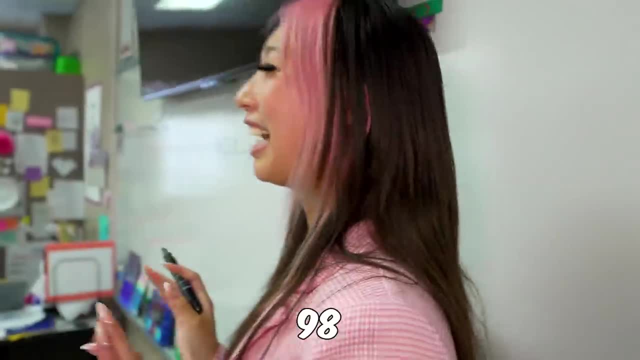 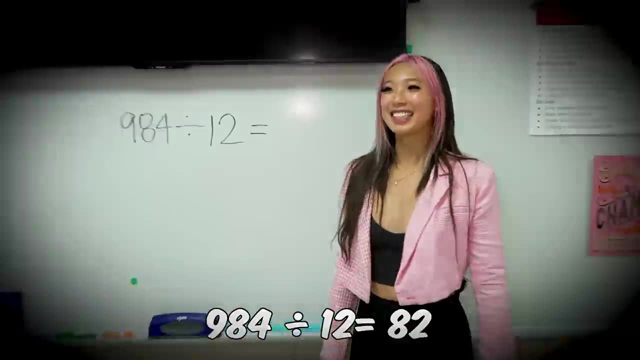 With team selected, it was time for the first problem. Okay, 984 divided by 12.. And the first problem got solved faster than I expected. All right, 82. 82?? That is correct. Do you guys want to come up here and show me how you guys did it? 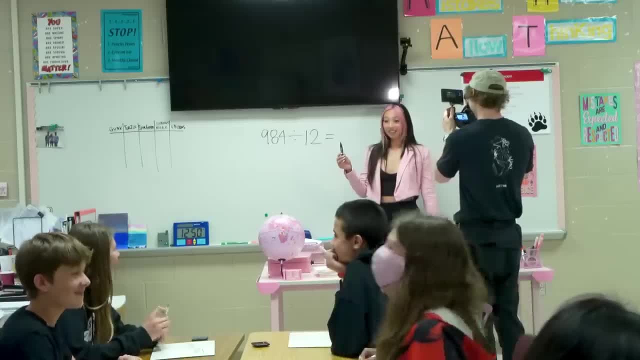 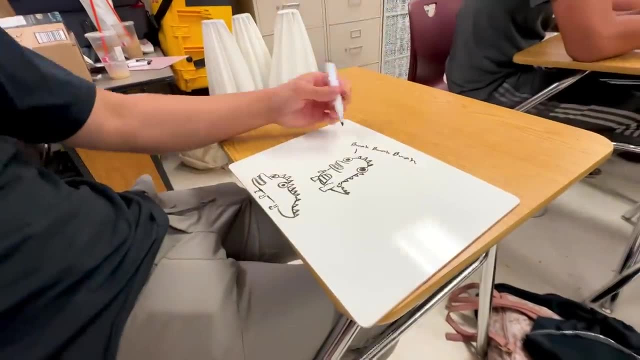 We used this calculator. Did I hear calculator In this munchie class? All right, I don't think that one counts. We don't use calculators in this class. Dude, you got the answer. I like that. With the calculator rule established, it was time to continue the competition. 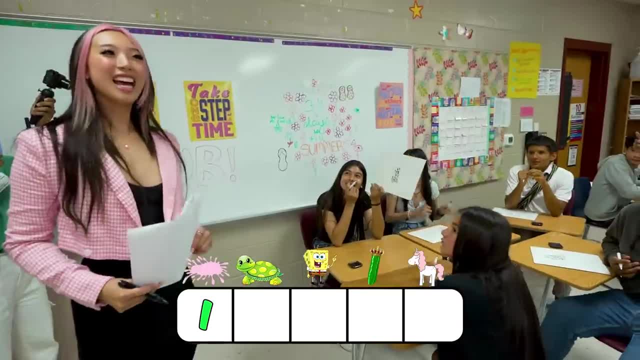 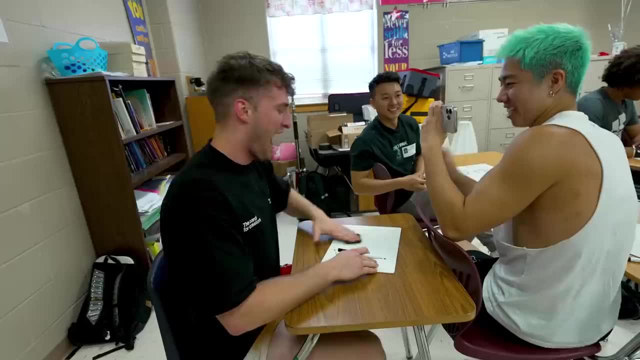 I gave the students another problem and another 516 plus 86. Got it Correct, But while they were answering the questions correctly, Jake was struggling. I got it wrong. I got it wrong. You were off by 400.. Jake, what's wrong? 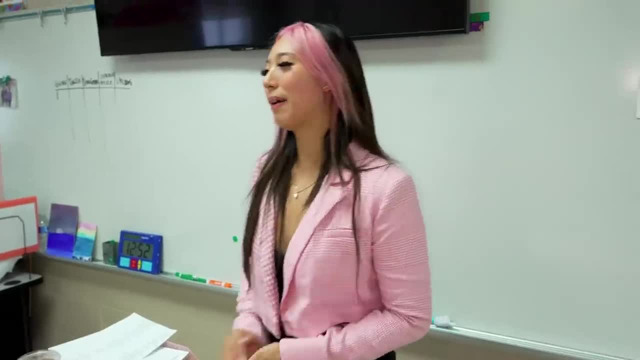 I got the wrong answer, okay. Is it hot in here? Do you want to come up and write your name on the board? This is all you guys' fault. All right, She's on my list. Jake, the seventh graders are laughing at you. 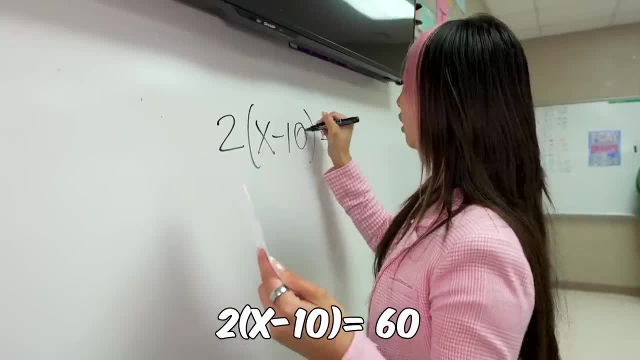 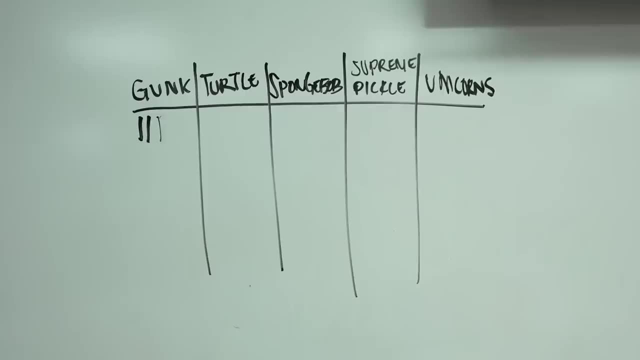 Yeah, This one is super fun. Show your work, you guys. One, two, three, four Guys, we got it. Is it 40?? Yeah, Before you know it, the contest was over. Team Guns got three points. 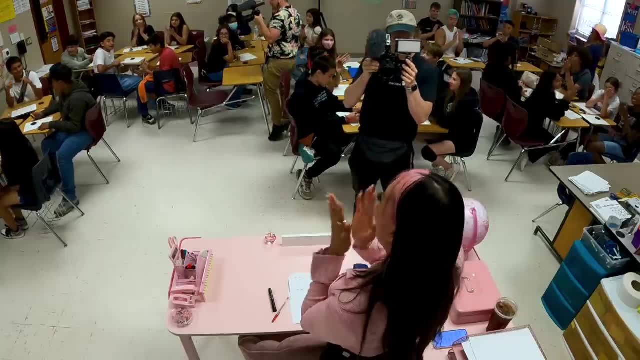 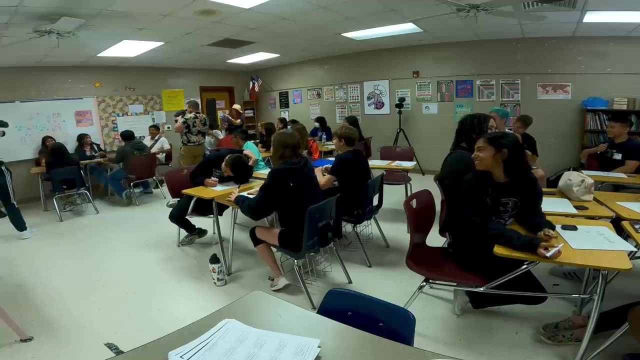 So everybody congratulate Team Guns for winning. Yay, And they all get a prize. You guys get to split $500.. Yay, If I want the students to pass the final exam, I need to make sure they finish it. So my next lesson was focused on speed. 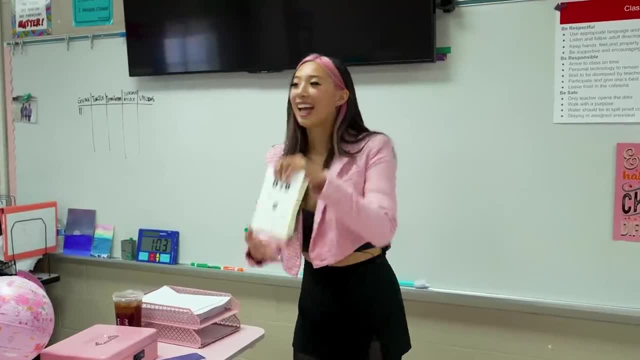 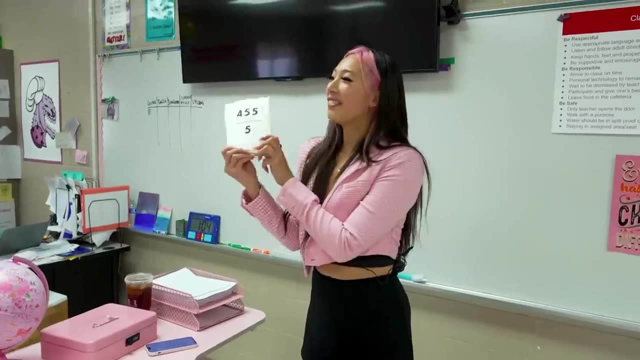 I'm going to give you guys flashcards. Answer as fast as you can. I test the division 828 divided by 9.. Got it Nice 92.. Nice 455 divided by 5.. Is it 95?? 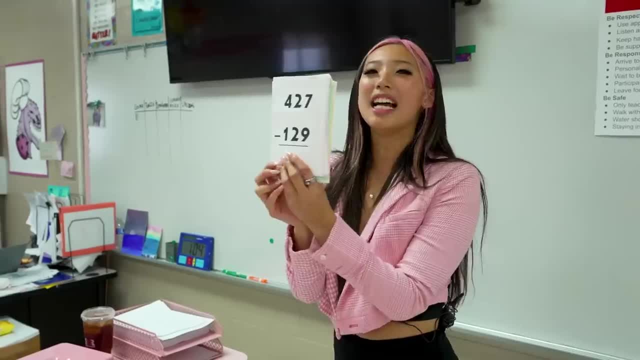 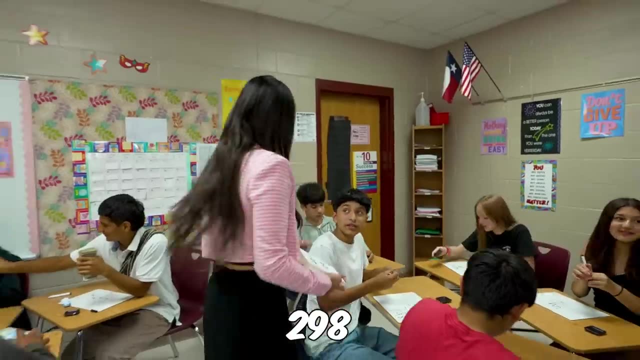 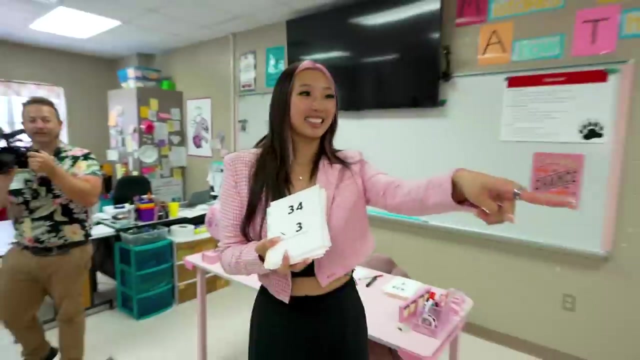 Yes, 91.. Yes, Subtraction 427 minus 129.. Oh, this one's a hard one, Nice, Nice. Yes, 99.. Yes, And multiplication 34 times 3. 4202.. Yes. 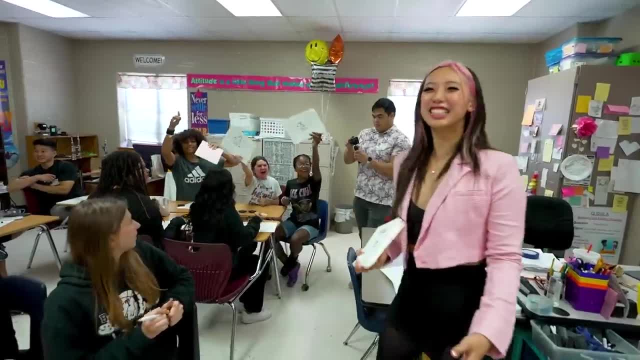 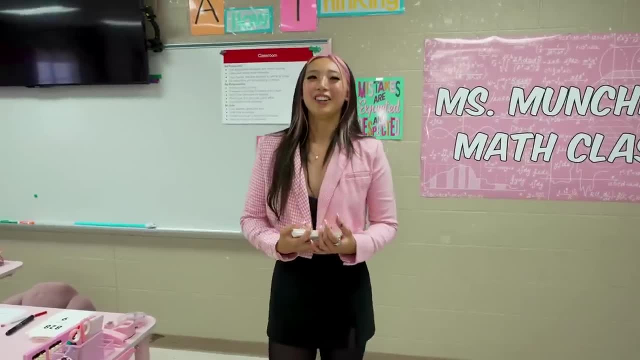 4202.. And the students were doing insanely well: Yeah, 102!. Yeah, But some still weren't participating. I couldn't leave anything to chance, So I decided to incentivize everyone to start answering. If you guys all get it right, I will tell a very embarrassing story of me in middle school. 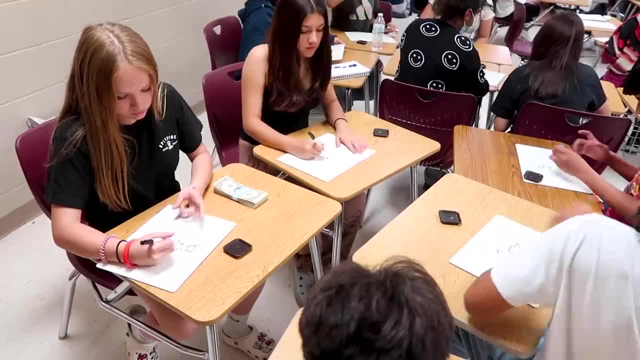 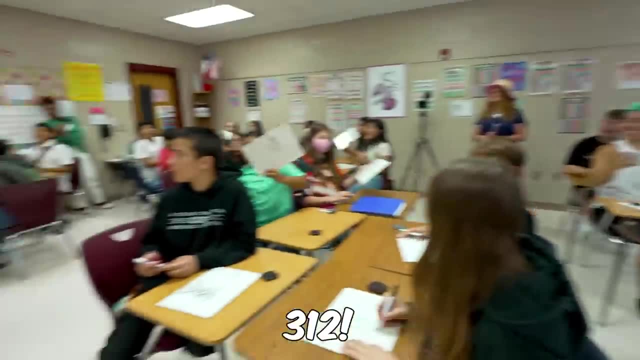 52 times 6. That was 30 of them. I've never seen them complete the problem so fast. I'm really curious for anyone to hear this story. What's the answer? 312!, 312!. Everyone answered, so it was time to spill the beans. 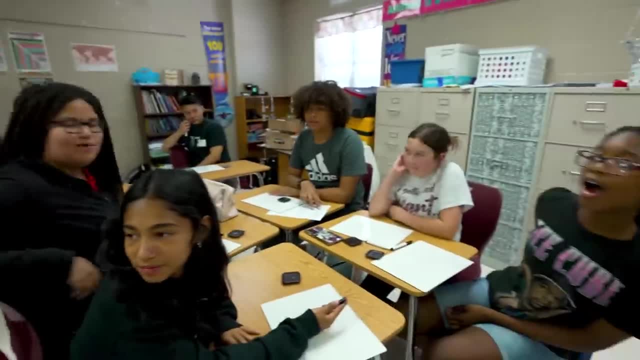 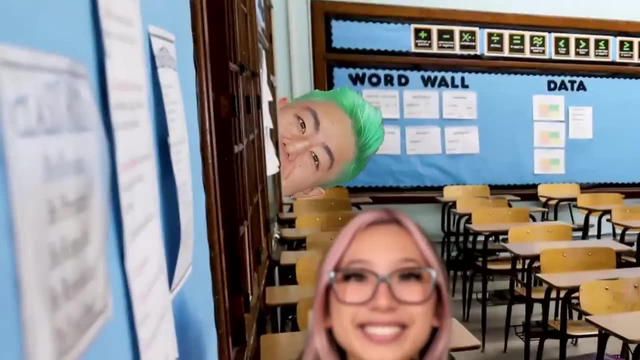 Do any of you guys have like crushes? Yeah, Okay, so everyone can relate. There was this really, really cute boy. That's me. I was in seventh grade. It was not you. Wait what No? 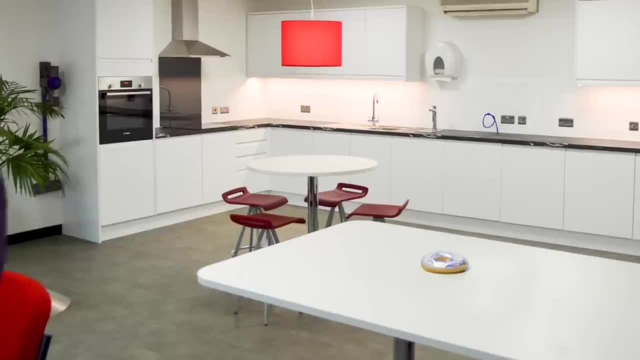 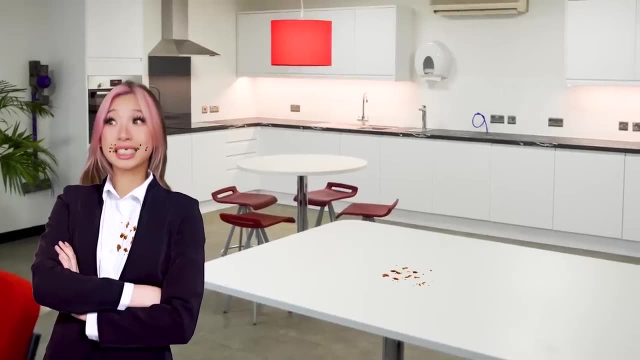 And I really, really liked him. I really wanted him to like. notice me. One day I had a donut- It was a chocolate donut, So I was so hungry so I ate it super, super fast. I had like chocolate all over my piece and all over my hands and shirt. 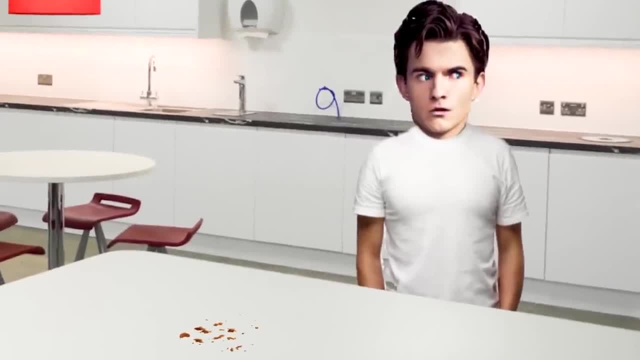 And the guy comes up to me and I'm like: oh shoot, I was just like hi, And he laughed at me and I never talked to him since. Good Lesson learned: do not eat chocolate donuts really fast. 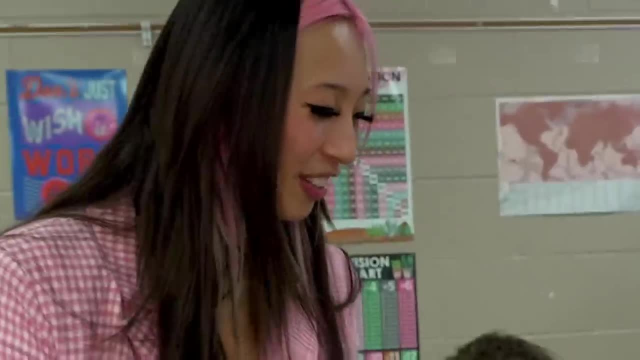 Hey, Michelle, I didn't know you had a crush before me. Yeah, I had crushes before you. Crushes, Yeah, With an S: Yeah. After reliving my childhood trauma, it was time to continue with the class. 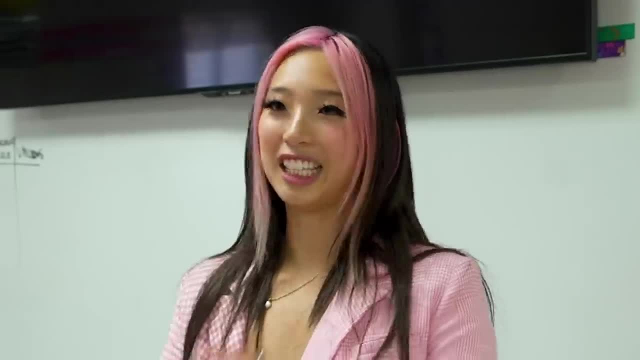 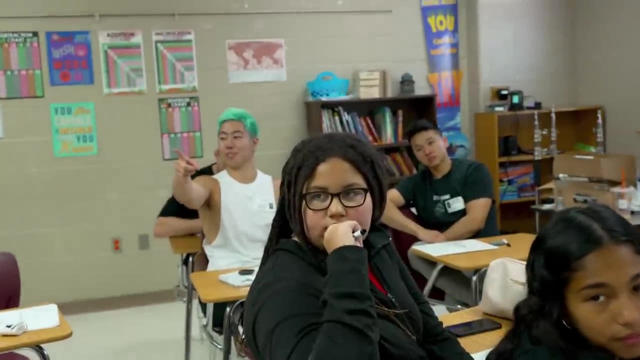 For my next game, I decided to increase the stakes. I'll give you guys a chance to win some money, but you guys have to try and beat me Like as a whole class, Whole class. Wait, you guys should test her to see if she's actually a human calculator. 86 times 94.. 8084.. 5,008.. That's a lot of bytes. 6,200.. 2,600.. 452, so 256.. 5,008.. 983 times 25.. 24575.. 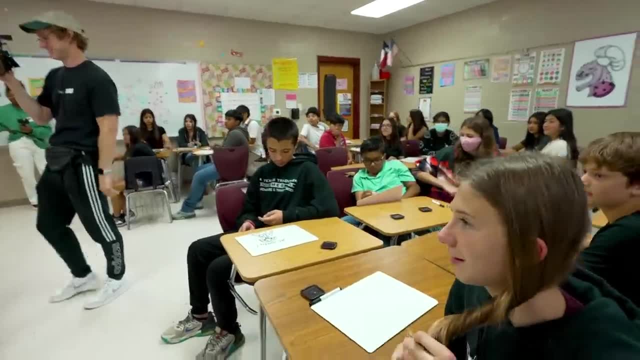 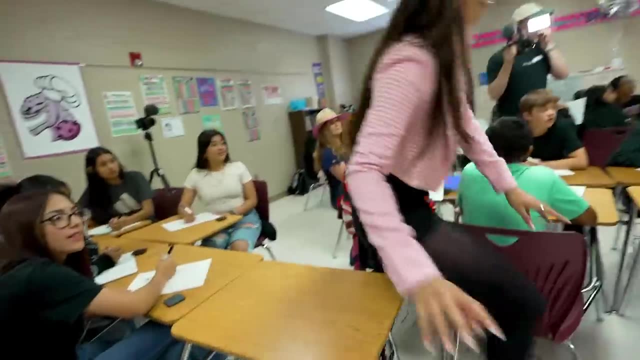 Well, good luck you guys. Don't let that discourage you. I'll give the class $1,000 if you guys can beat me. No calculator. My teacher assistant will be watching, Ready and go. Oh my goodness. 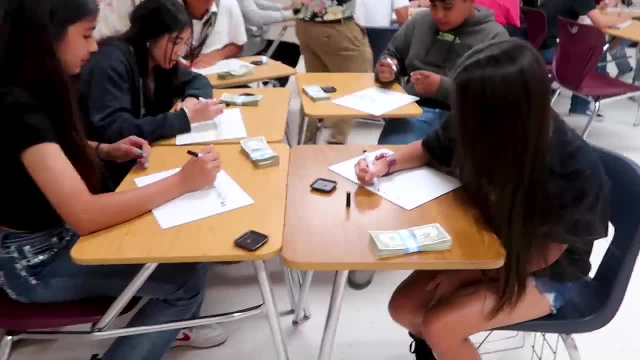 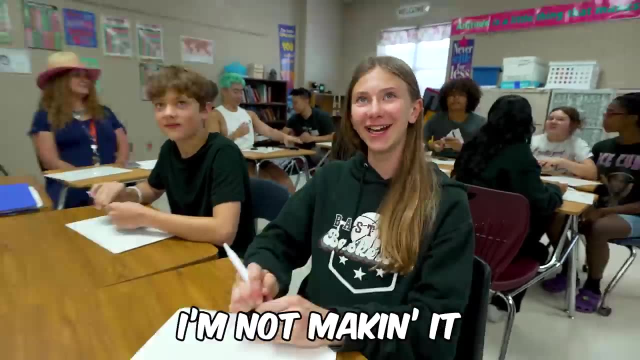 How is she doing that? That's right, She's done. Sorry guys, I've been discouraged. I'm not making it through high school. I didn't have any hope. I have no words. The kids weren't feeling very confident after the competition. 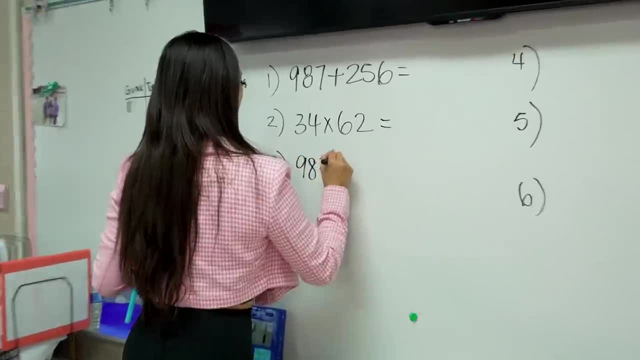 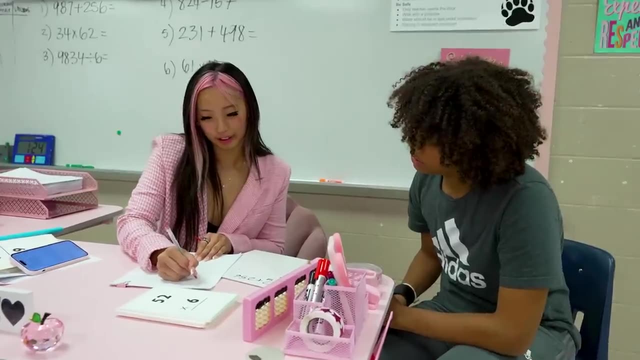 With the final test just around the corner, I decided to give them a few more practice problems to get them as ready as possible. Good job everyone. I even helped some kids out one-on-one. So then I do three over here and a one over here. 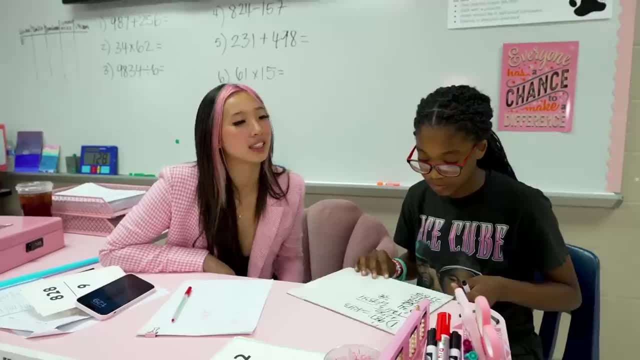 So this is the answer, Thank you. What's 38 divided by six? I don't know. There's six, then you add six, then it's 12,, then 18.. So it seems like 36 is the closest. 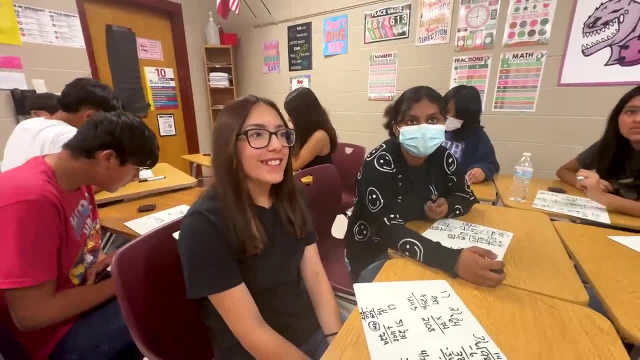 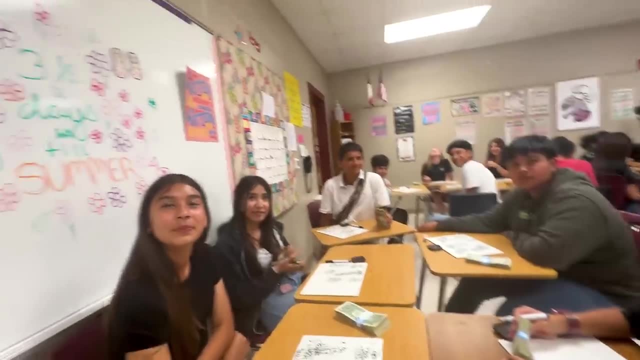 And under 38,? the answer is six. Do you think Michelle's a good teacher? She's pretty and she's good at everything, Very smart. Yeah, she's really pretty, She's really really good. What I'm hearing is: you guys like her as a teacher because she's smart and pretty. 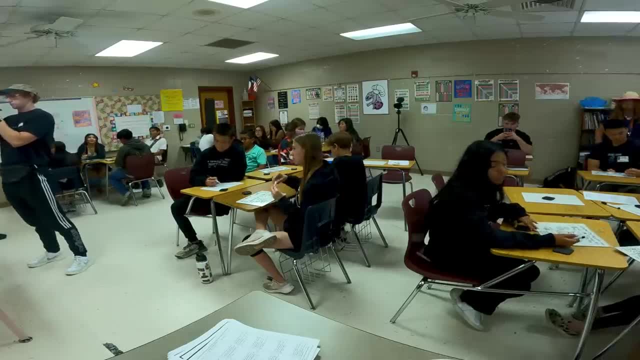 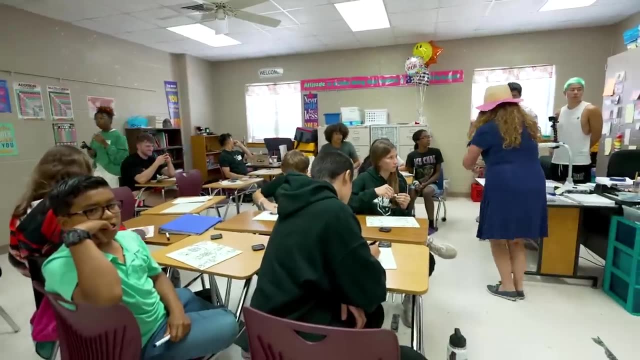 Yeah, How did everyone feel about the practice round? Easy, Easy. With our last practice round over, it was time for the test. I really hope everyone passes, because I do not want a tattoo. Everyone just do the first five problems.